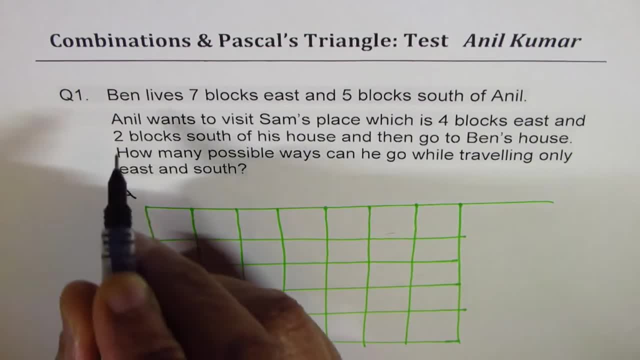 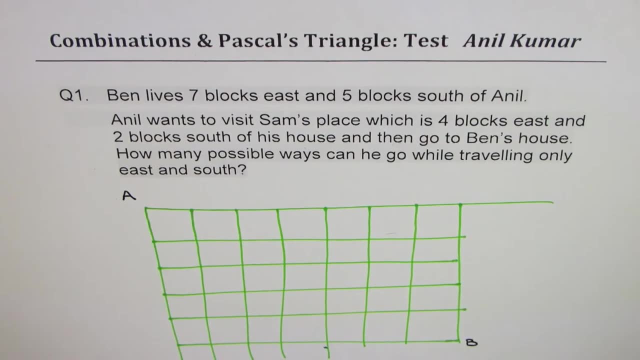 from here. Let us say Anil starts from here. Ben lives seven east and five blocks south. So this is Ben B. Now here we have a condition which says Anil wants to visit Sam's place, which is four blocks east and two blocks south. So that means one, two, three, four blocks east, one, two. So 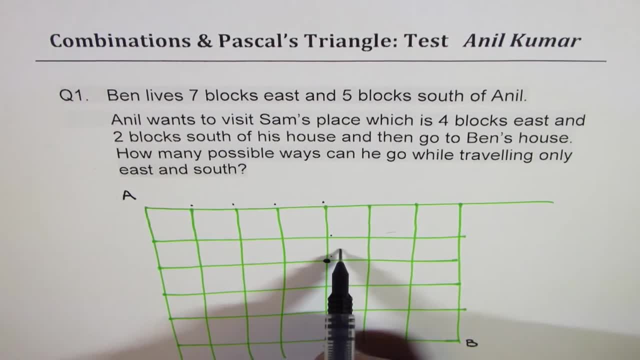 that place. So Anil wants to visit Sam- Let's call this S- and then go to Ben's place. Now, if that is the condition, then how many total possible paths are there? That is the question for you. So I'd like you to pause the video, answer this question and then look into my suggestions. Now let's begin. 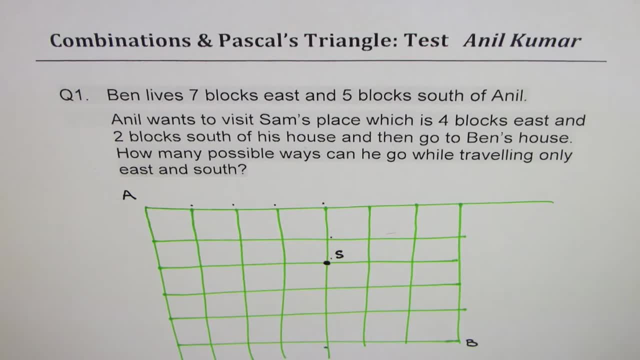 by counting the number of paths. So if we go only east, let's be one, one, one, one. then Anil has to turn, So that means one likewise, come In this direction, one and one. Since Anil can only travel east and south, we kind of stop here, right, And 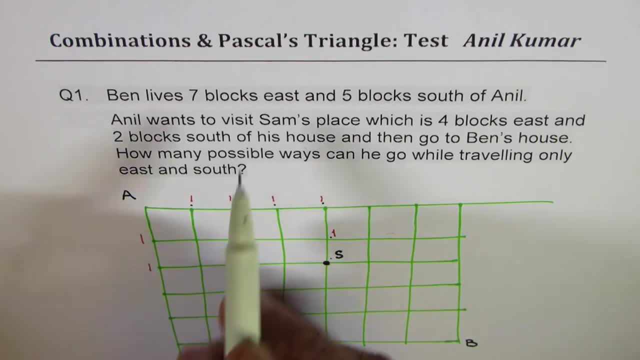 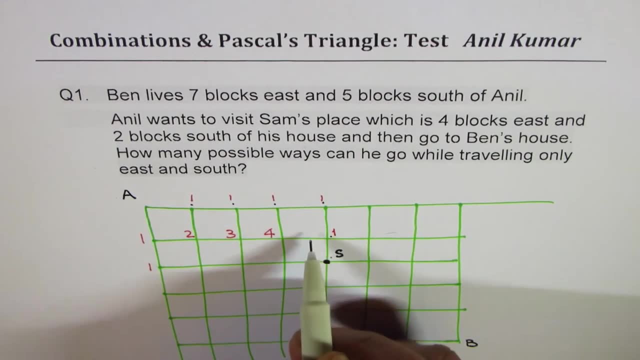 now let's see the possible paths and combination using Pascal's triangle concept. So one plus one is two, two plus one is three, three plus one, four, four plus one, five. right Now, this way, one plus two is three, three plus three, six, six plus four, 10,. 10 plus five is 15,. 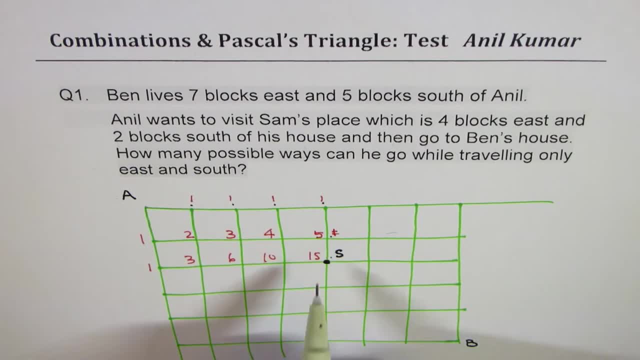 right, Okay, Now from here. now he has to depart to get to Ben's place. So from here going east will be 15, 15 and 15.. And south also, if he continues to go south, it'd be kind of 15, 15 and. 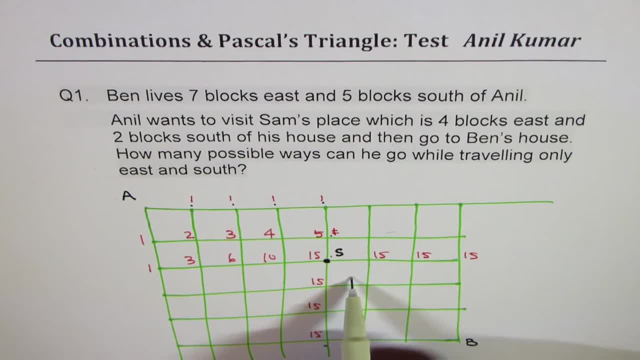 15.. But this way we get more number of paths. 15 plus 15 is 30,. 30 plus 15 is 45.. 45 plus 15 will give us 60.. Adding these two will give us 45,, 45,, 45 is 90,, 90,, 60 is 150.. And then here we get 45,.